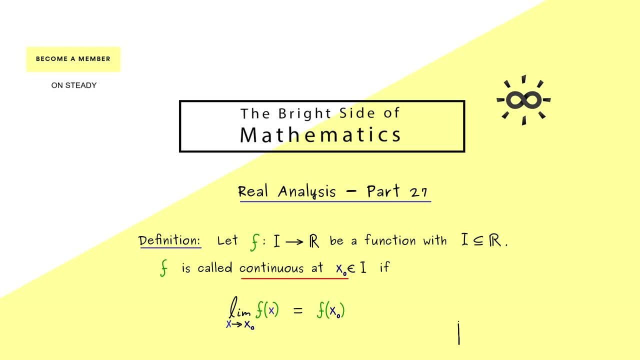 of x0.. Here it's important to remember that this is indeed a local property. This means that if you have a graph like this, you would fix a point x0 and you would zoom in at this point and look what happens. Also, you already know, in the definition of the limit we have two directions. So what happens? 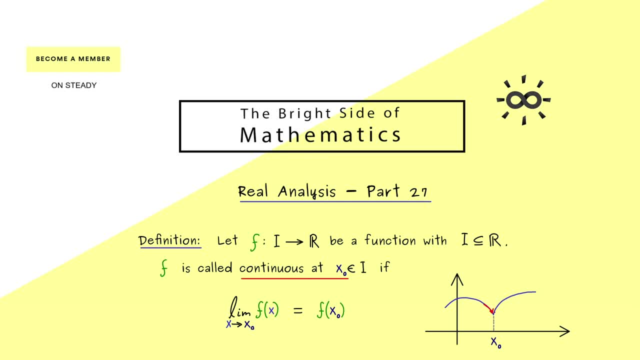 when we come from the left hand side, and what happens when we come from the right hand side And when both approximations go through the value. at this point we say that the function is continuous. at this point, So for this definition it only matters what the function does around. 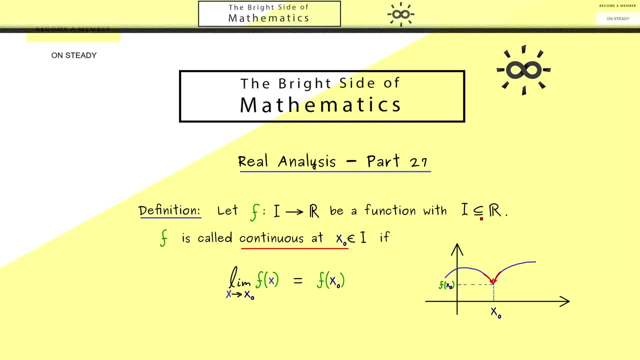 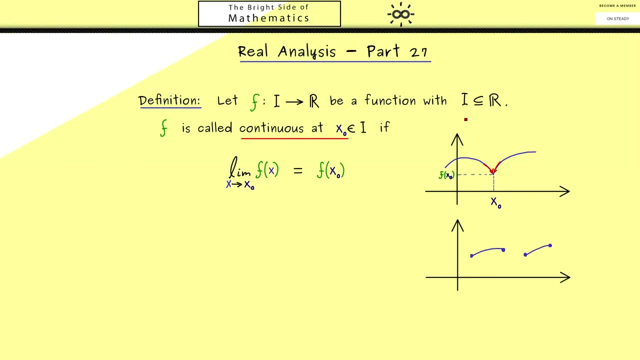 this point And for this reason we have to talk about a special case that can occur. Of course, it can happen that the domain i is not an interval. This means there could be some holes in the domain of definition. Therefore, for example, at this point we only would have the right limit. 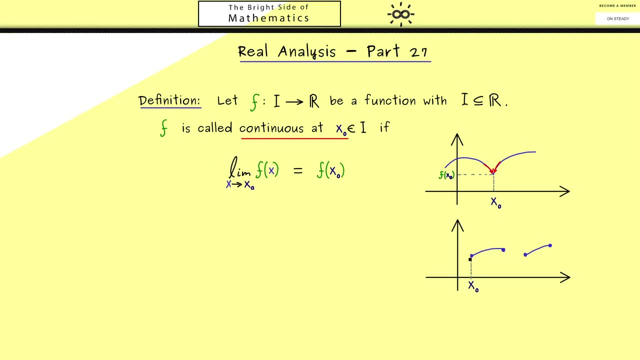 Which is of course, not a problem, because the whole limit still exists. It just gets simpler because we only have to look at one direction. However, what happens when this direction also does not exist? In this case, the limit symbol here does not make any sense. 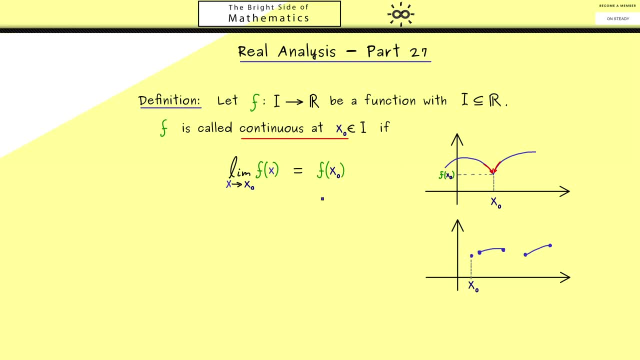 Hence, for such an isolated point in the domain i, we need another definition. Now, here, please recall, continuity should exclude jumps we could have in the graph. And of course, for such an isolated point here a jump in the y direction can not happen. Or in other words, when you zoom in at this point there is nothing around. Or to put it in other: 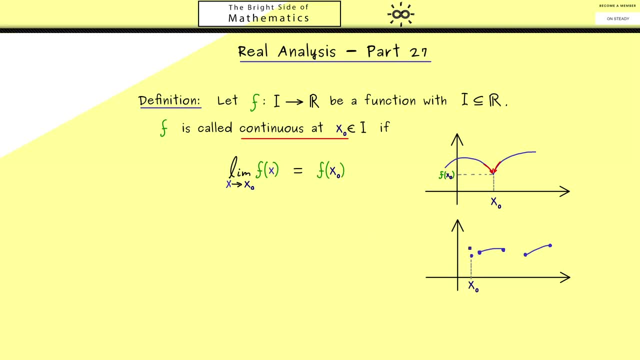 words. if you zoom in at this point you see there is nothing around this point. Therefore, for such we also call the function f continuous at this point Here. isolated in i just means you don't find a sequence xn from the outside, such that the limit of the sequence is x zero. 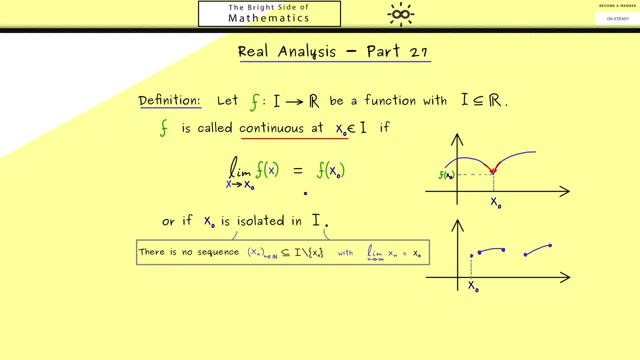 However, still the important case is that we have a point that is not isolated such that we need this condition here, And with this we have the whole definition for f being continuous at a given point, x, zero, And now we can simply extend this definition. 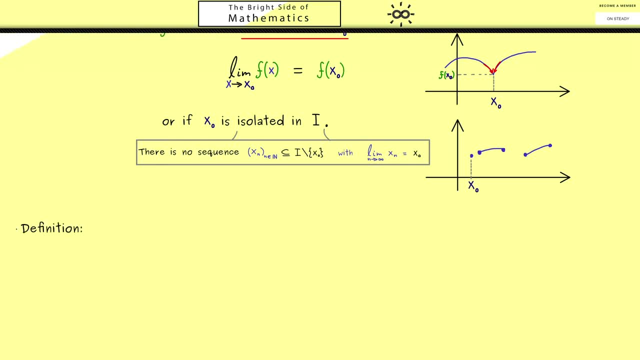 to all points in the domain i. This is a common procedure to make a local property global. Now a given function, f, is simply called continuous or if you want to emphasize the domain, you would say continuous on i, if f is continuous at all points in the domain i. 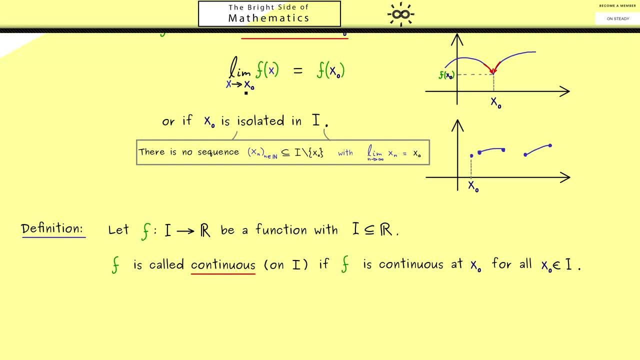 So the property from above holds, no matter which x zero you choose. Therefore, an important thing to remember is that continuity helps you when you deal with x zero. This means that if you have such a limit, you can pull the limit symbol inside the function. 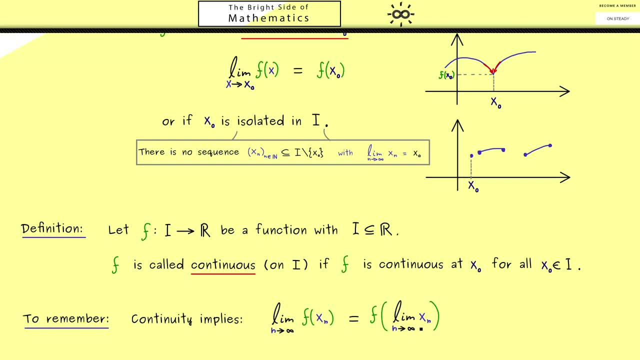 Of course, you also have to put in that this limit exists and lies in the domain of f. However, in this case, the continuity of the function f tells you that this operation here is allowed. Ok with this, i think we are ready to talk about examples. 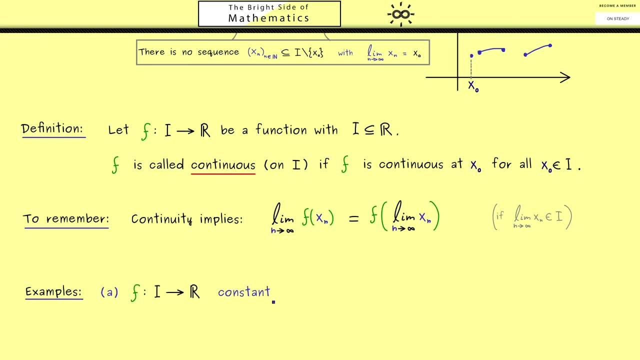 Let's immediately start with a simple one. If we have a constant function, no matter what the domain is, it's always a continuous function. This is not hard to see, because the sequence of the values is always a constant sequence. Now, if we manipulate this example a little bit, 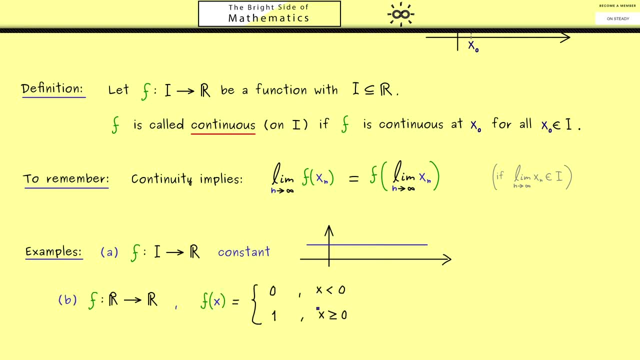 we get a function that is not continuous. So here we have two constant functions that we put together, Which tells us that we here have a jump at zero Because the left limit is different from the right limit. Therefore the function is not continuous at the point zero. 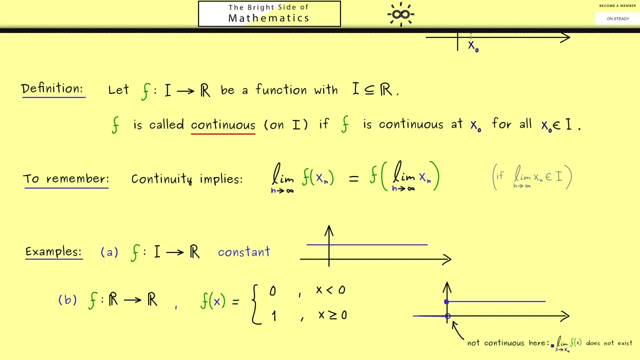 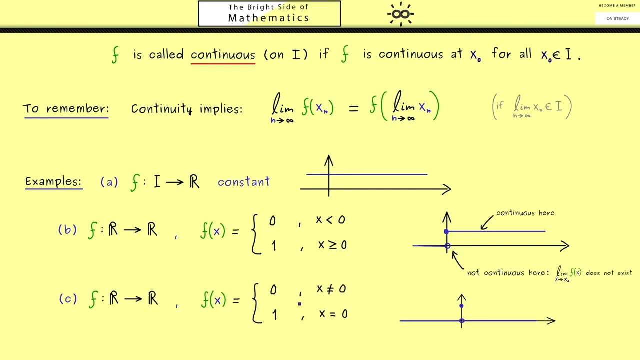 The problem is simply that the limit at this point does not exist. However, at any other point we don't have this problem. Hence we have continuity everywhere else except at zero. Ok, next, let's look at a similar example. Here, we just change the value zero at one point. 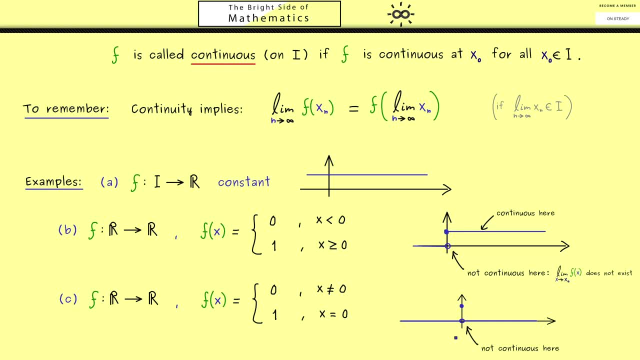 And we already know this from the last video. Therefore, we already know the result here. It's not continuous at the point zero. You already know that. You already see the jump here. However, now the limit exists at this point, but it's not the same as the value at the point zero. 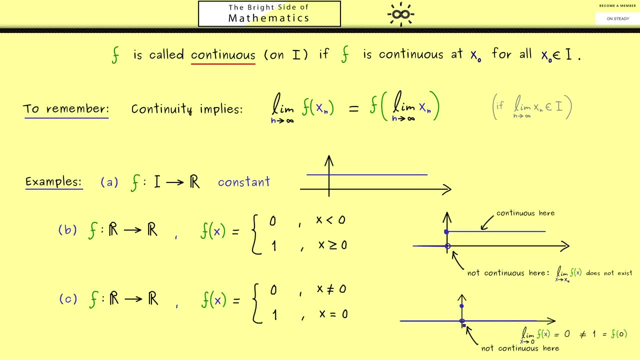 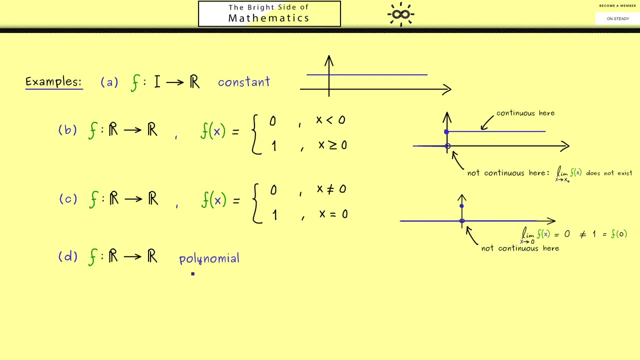 But still the result is it's not continuous at the point zero, but everywhere else. Ok, let's also recall a positive example from the last video. This is just a general polynomial which can be defined on the whole real number line And it can be written in this form: where we have coefficients a, k, 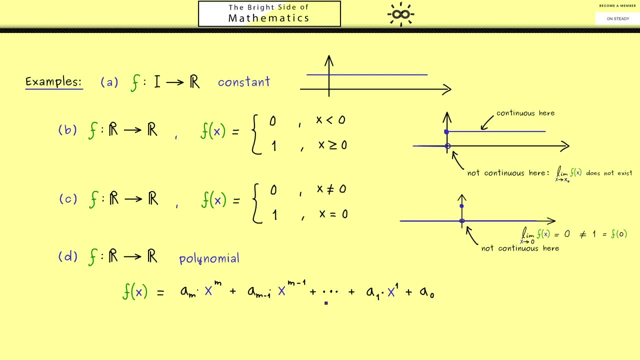 And now you know that we have already showed, by using the limit theorems for sequences, that we have continuity at all points. Or, more explicitly, we have shown that the limit x to x zero is the same as f of x zero. Therefore, such a polynomial never has jumps. 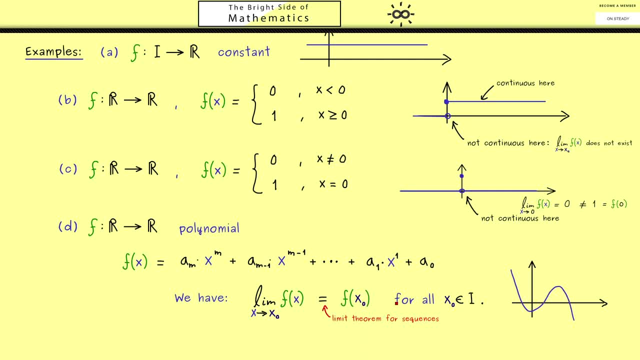 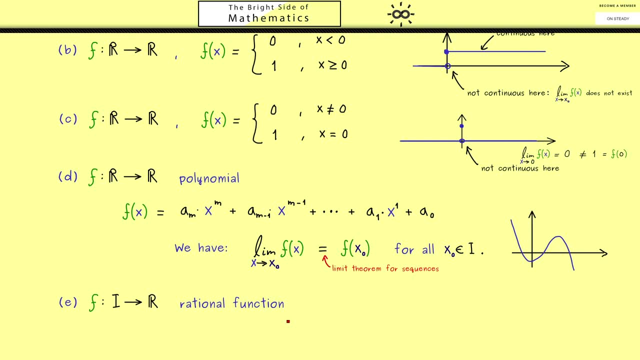 So this is a very nice and important example of a continuous function. A straightforward generalization of such a polynomial is a so called rational function, And it is also a continuous function Everywhere where we usually define it. The definition is simply given by a fraction, where we have one polynomial in the numerator. 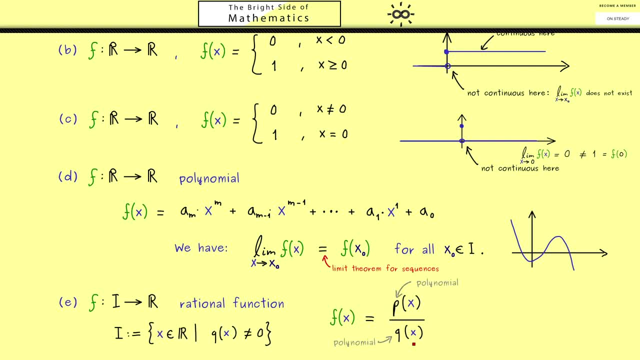 and another one in the denominator, And for this reason, in the domain of definition we have to exclude the points where q of x is zero. However, then we get out a nice continuous function. Indeed, it's not hard to show the equality here. We just have to use the limit theorems again. 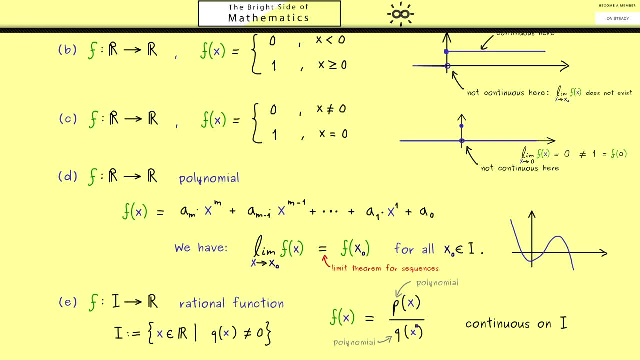 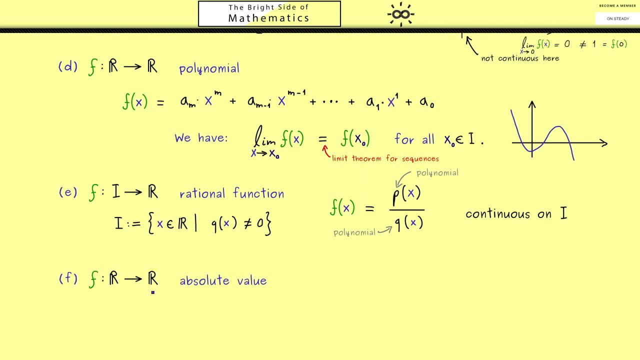 Because we have one limit theorem For sequences that considers a quotient. Ok, maybe at this point it might be helpful to look at a very concrete example. What we can do is to look at the function given by the absolute value. So we know, by definition, the absolute value is given by two cases. 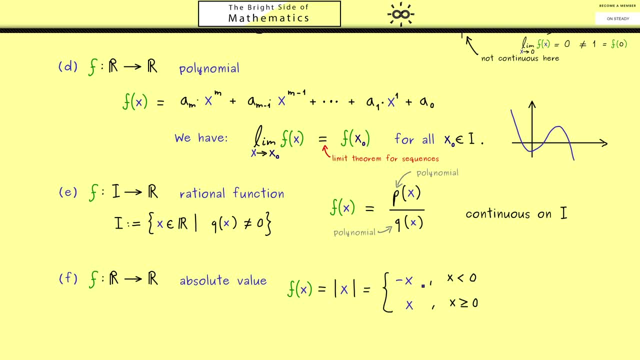 For positive numbers we don't change anything, And for negative numbers we change the sign And of course, zero stays at zero. Therefore the graph of the function looks like this. So you see, For every point except zero, continuity is clear, because there it's simply a polynomial. 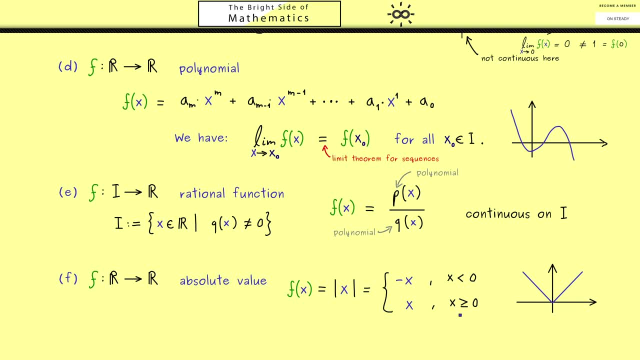 There, we just have to consider minus x or, in other cases on the right hand side, just x. However, for the point zero, we have to consider both cases at the same time. Therefore, let's calculate the limits First. let's consider the left limit when we come from the left hand side. 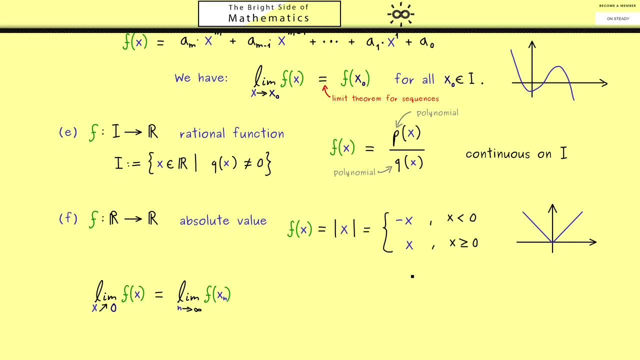 So we consider a sequence: xn. that is always less than zero. Therefore we are always in this first case. so we can substitute f with minus x, And then this limit is easy to calculate, it's just zero. Then in the next step, of course, the right limit has a similar calculation. 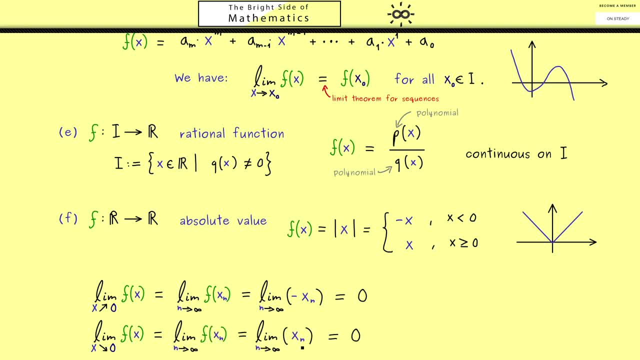 There we can substitute f with just xn. Both times we get zero. therefore, the limit exists with value zero, Which is the same as f at the point zero. Therefore, the result is: the absolute value is a continuous function. Ok, now for the last example. we should choose one that is not continuous. 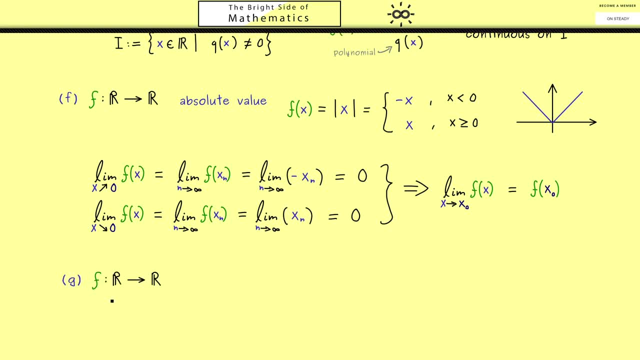 It's also easy to define. but what we get is that we don't find any point where the function is continuous. So we put the function to one when x is a rational number, and otherwise we put it to zero. So what you should immediately see is there are a lot of jumps involved. 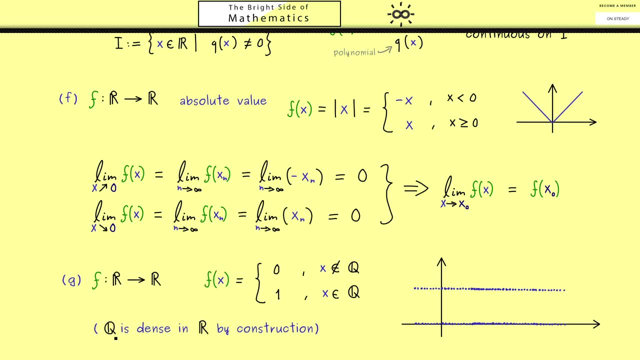 Now, an important fact we can use here is that q is dense in the real number line, And this is indeed what we have by construction of the real numbers. However, of course, the only thing we need is the meaning of this. It tells us that every real number can be approximated by a sequence of rational numbers. 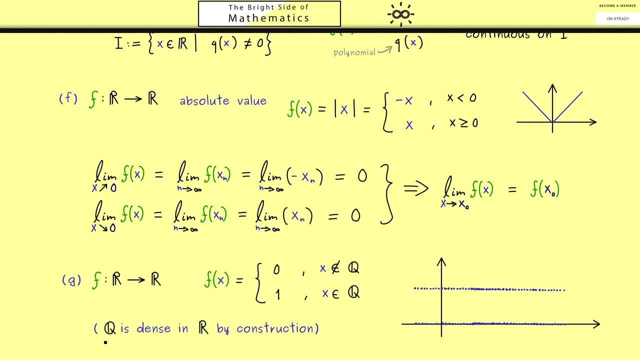 So for any real number you can take a sequence of rational numbers where the limit is this real number, And indeed the same works with sequences, with irrational numbers. And exactly for this reason this limit here does not exist, Simply because you can take a sequence that stays at one the whole time. 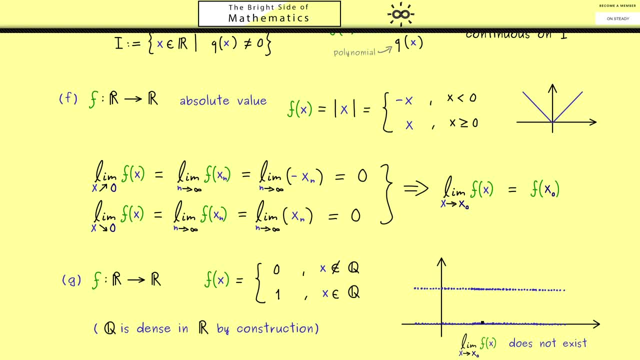 And you can take another sequence that stays at zero the whole time. Therefore, we can always produce two different limits here. So here we have an example that is at no point continuous, Or you could say: it's everywhere discontinuous. So please keep that in mind. Continuity is a special property and not all functions have it.